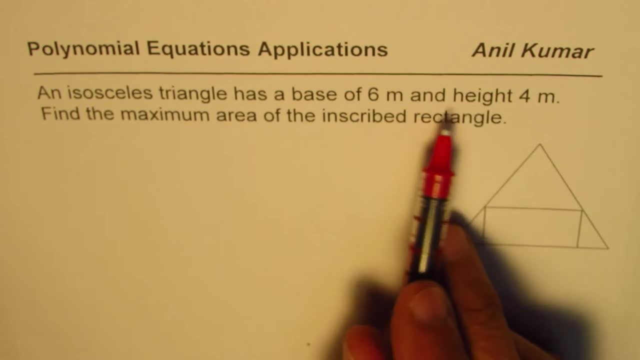 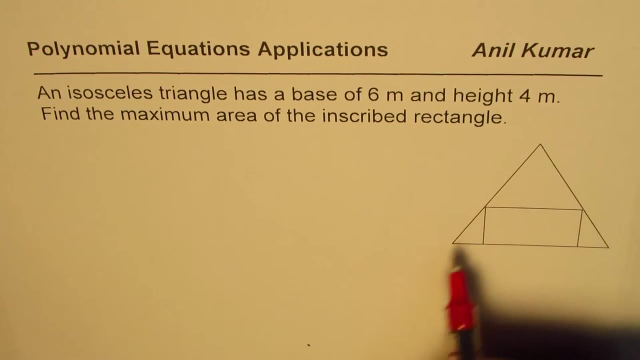 triangle has a base of 6 meters and height 4 meters. Find the maximum area of the inscribed rectangle. So we are given an isosceles triangle that means two sides are equal and that is the inscribed rectangle. We need to find maximum area of the rectangle that can be inscribed within. 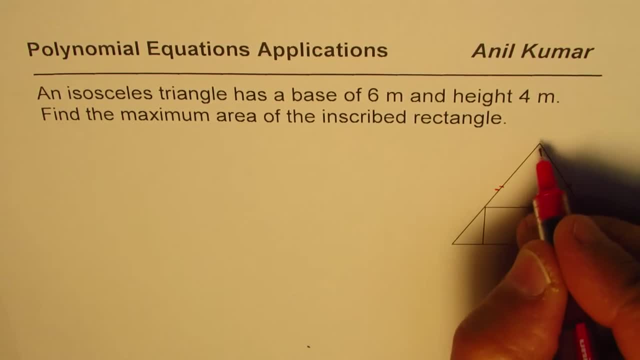 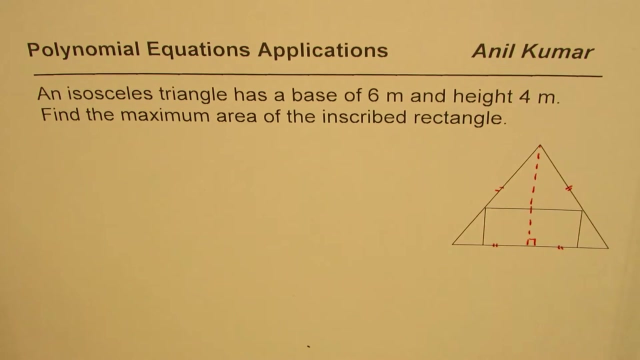 this triangle. To begin with, let me drop a perpendicular from the vertex right. So I'm just dropping a perpendicular. Since this is isosceles triangle, this perpendicular is going to divide the base into two equal parts, right? What are we given here? We are given that. 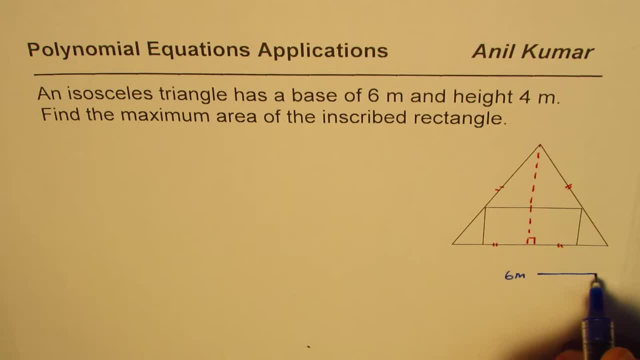 the base is 6 meters, so we are given this is 6 meters, right, and the height is given to us as 4 meters. Let me write down here: the height is 4 meters. We need to find maximum area of this rectangle. So let us assume that. 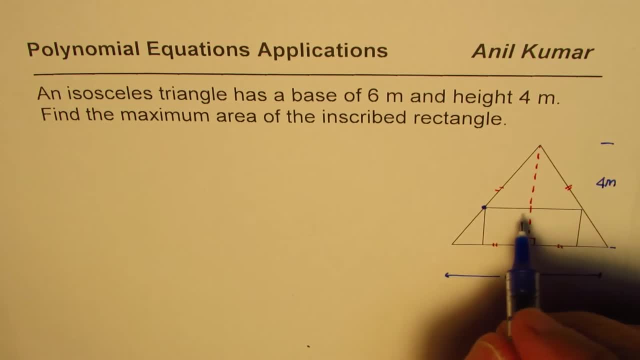 a point here is: or let us say the dimensions of this rectangle are length be 2x, So x this side and x this side. So let us say the dimension of the rectangle is 2x, that's the length, and let the width be y. So this width be y, Let us assume that. So what we have considered here is that rectangle. 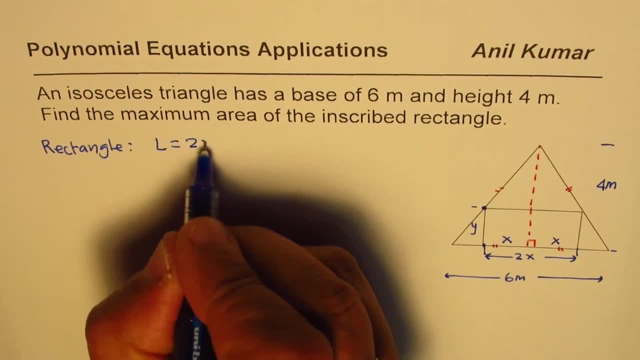 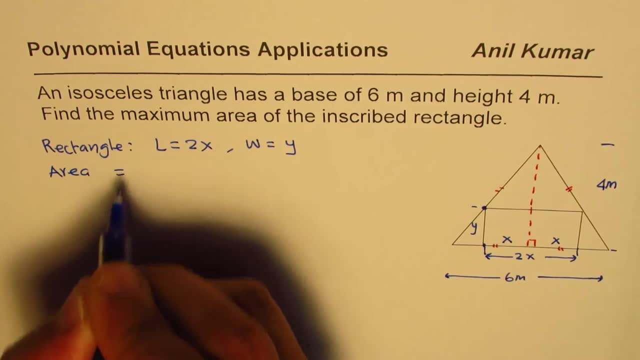 as length equals to 2x And width equals two y right. So in that case, area will be equal to length into width right, length into width. That means 2 x times y. So that is going to be the region. We need to maximum this heraE. Now, to maximize, we have two variables. we should write these variables In terms of one another So that, in terms of this presidency, we can writeuest failing variable. we should write this variable unexpected. 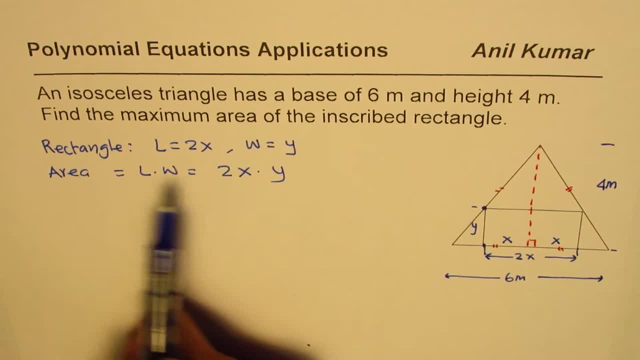 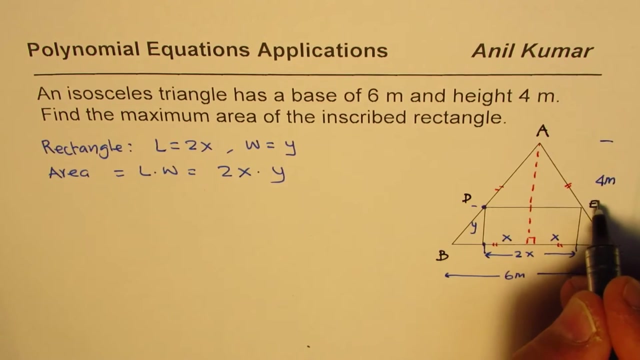 we could write equation of area in terms of one variable. So that's the whole idea. How can we do that? Well, we can do with the help of similar triangles. Let me label this triangle. Let's say this is ABC. Let's call this point as DEFG. More important for me are these two points, right So? 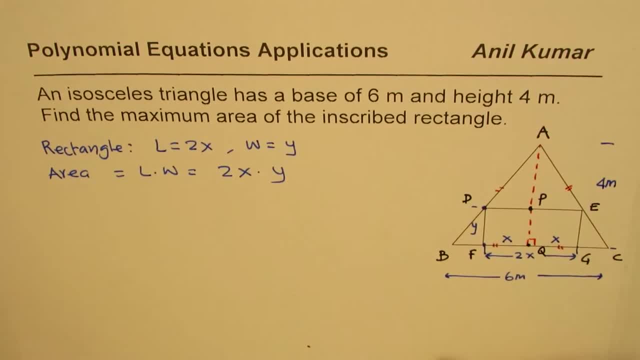 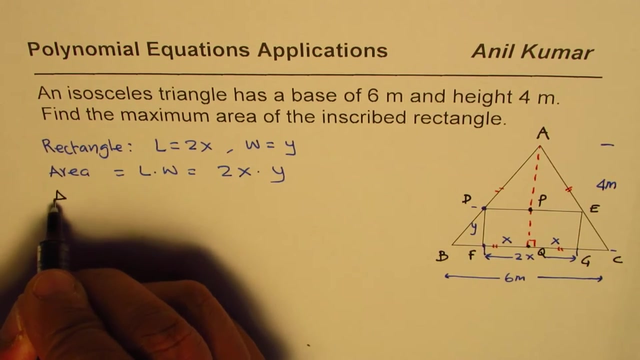 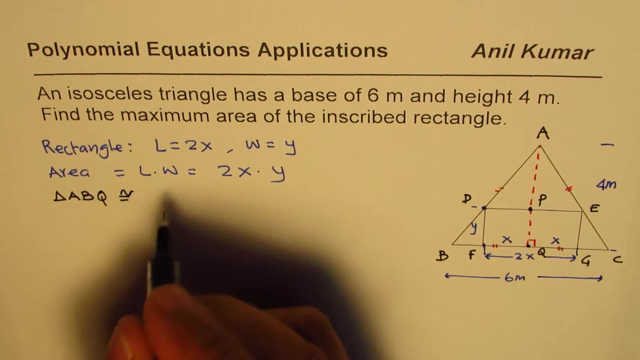 let's make them P and Q. Okay. So what do you notice here is that this big triangle ABQ is similar to the small triangle ADP. So what do we notice here is that the triangle ABQ is similar to the triangle ADP. 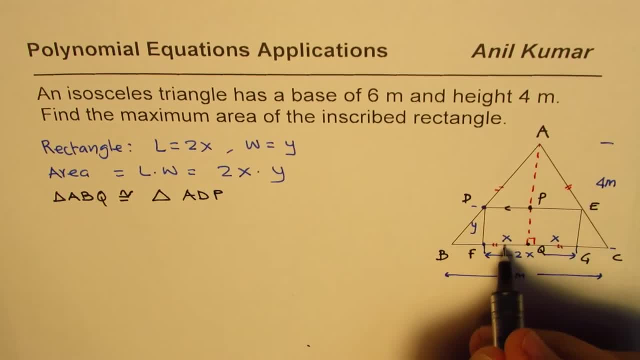 Since this is a rectangle, the sides are parallel, correct? So the angles are the same and that is 90 degrees. this is also 90 degrees, correct? So we have from two ways. These two are similar triangles. since they are similar triangles, ratio of these sides should be same, right? 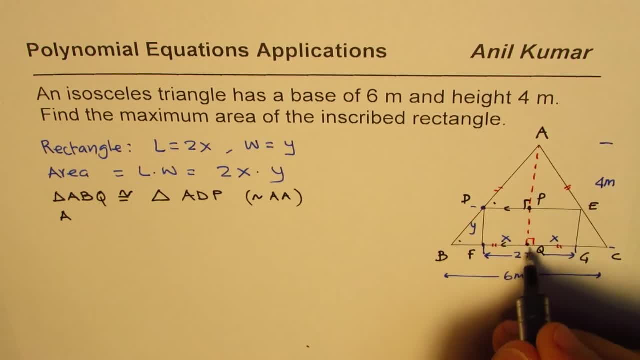 So we can write that AQ over BQ should be the same Red, mientras que BQ versus BC versus AMBQ, boobs together should be 90 degrees角. So we have So from these two ways. another way is to write AQ over BQ. 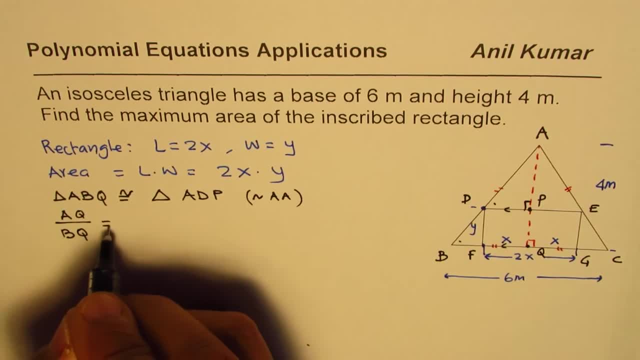 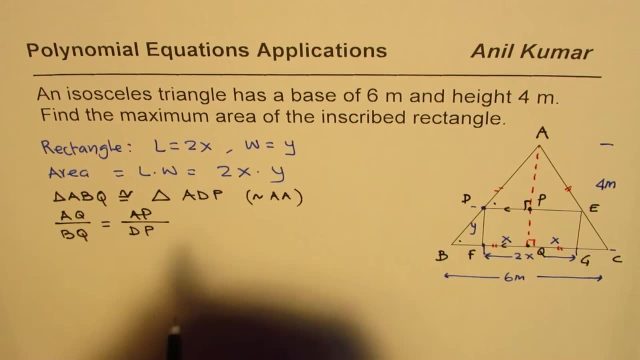 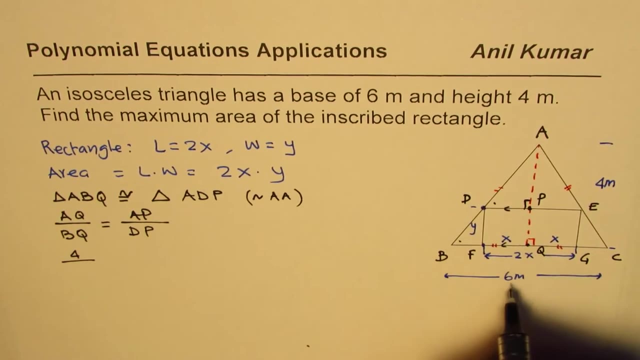 over BQ should be equal to a p over d p, right over d p. now, what is a q? a q is given to us as four meters, so i write four. b q is half of six, so right, so this is three. b q is three for us, so that is three. 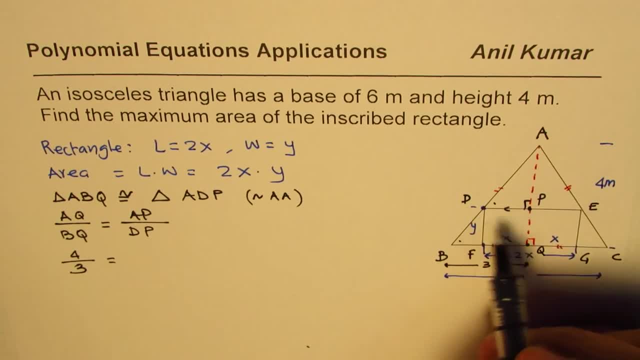 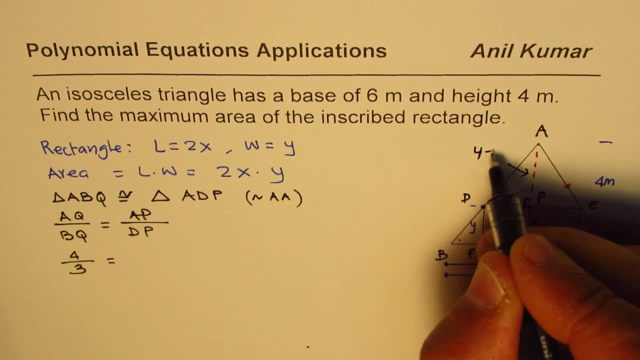 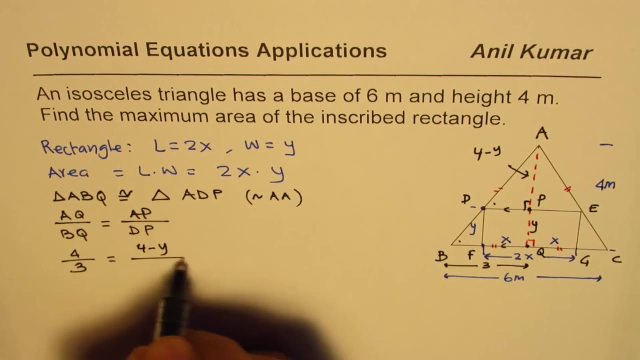 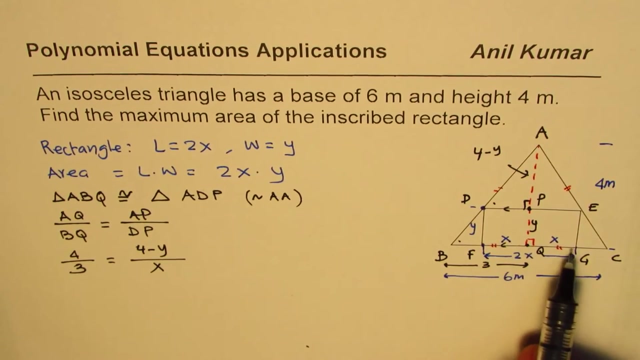 for us: a p, a to p. since this height is y, a p will be four minus y. so this height will be four minus y, since y is the width of the rectangle. is that okay? so a p is four minus y and d p is x for us. okay, we have taken length of the rectangle as two times x. 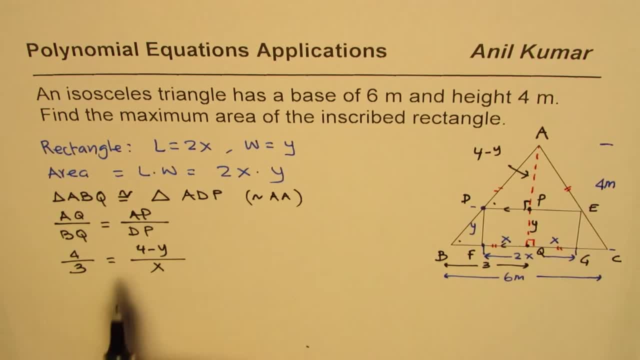 from symmetry: x on this side, x on the other side. now this equation helps us to write x in terms of y, So we'll cross: multiply: x equals to 4 over 3 times 4 minus y. Do you get it? So we got x in terms of y. Now let's get back to the original equation. 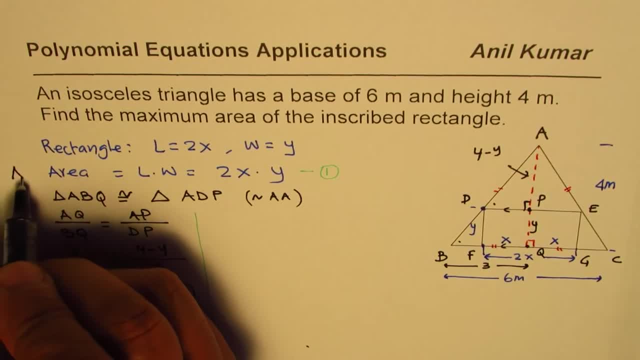 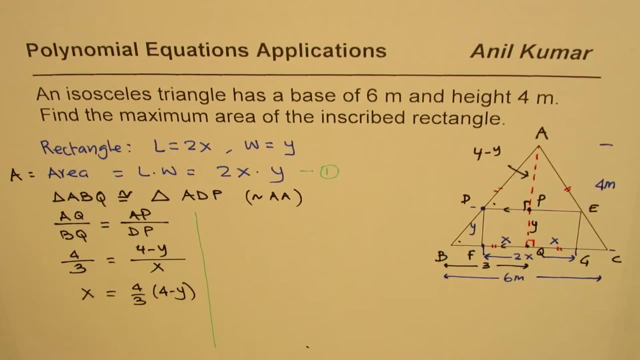 Let me write this as equation 1.. So area- we're saying area- is equal to this. I'll replace this x here with this expression of x. Let me call this as our equation number 2.. Okay, let me write this as equation 1 and this as equation 2.. Okay, so we'll sub equation 2 in 1.. So what do we get? 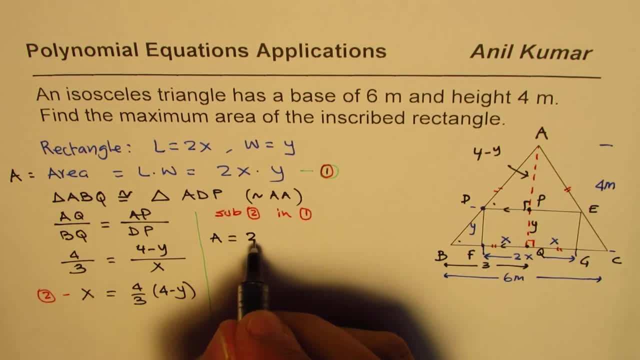 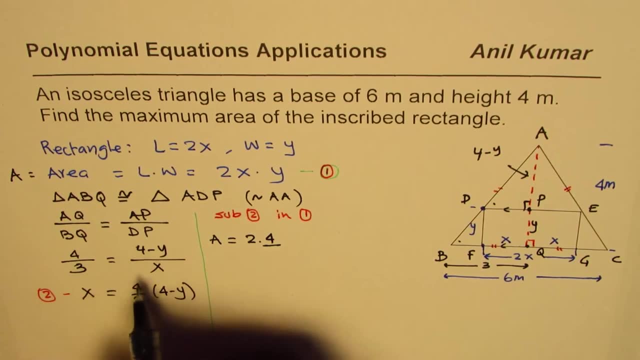 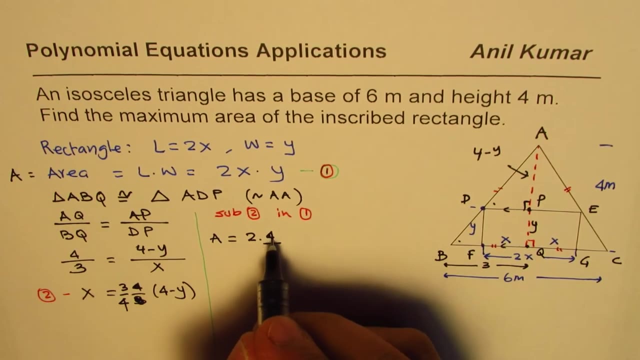 So we get area as equals to 2 times x. value is 4 over 3.. I'm sorry, when we cross multiply it should have been 3 over 4.. Let me change. So when you cross multiply it should be 3 over 4, right, I did a mistake. So it is. 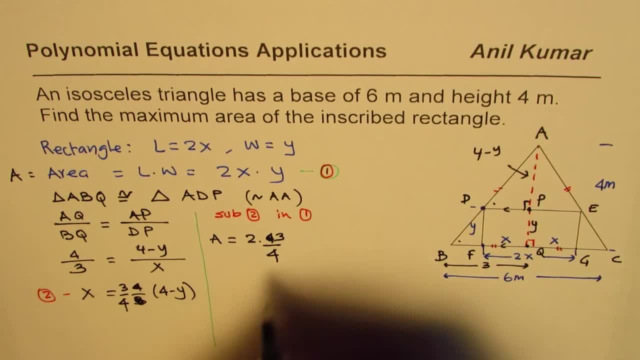 3 over 4, right times, 4 minus y. So that is the x value and we have y also here, So y. So that becomes the area. Now this area is in terms of y, So I could also write this as: 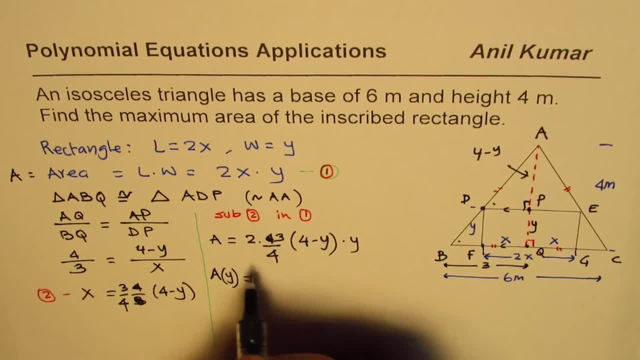 a as a function of y. Do you see that? Now? let me divide this, simplify it a bit. We get 3 over 2 times y Times, 4 minus y. Is that okay? So that becomes the area. We need to maximize this area. 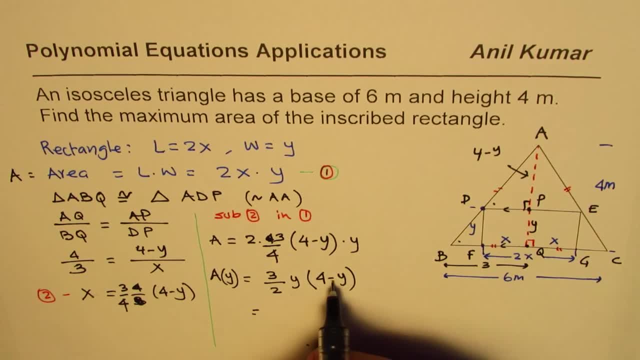 Okay. So you will notice that if I take minus common, I get minus 3 over 2y times y minus 4.. The only purpose to rewrite this equation with minus here is to remind you that it is like a parabola right. It is like a parabola right. It is like a parabola right. It is like a parabola. 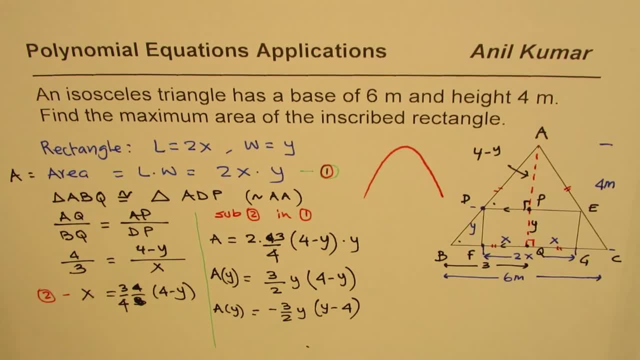 opening downwards, Do you see that Where it has two zeros, correct? And those two zeros are where Zeros are at 0 and 4.. So let me just kind of make a sketch for this parabola. So 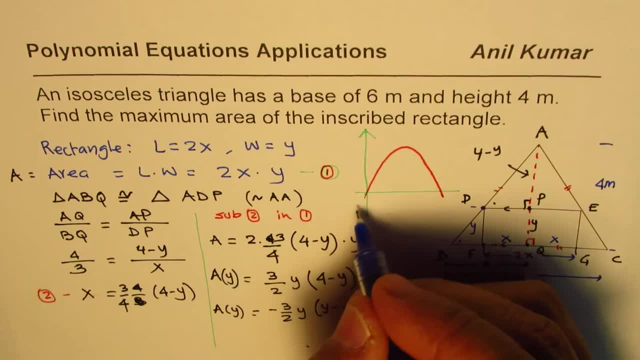 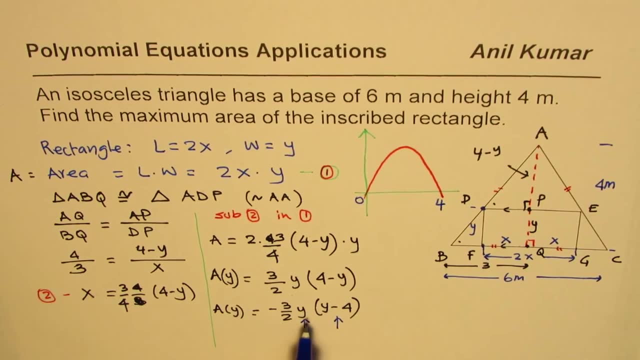 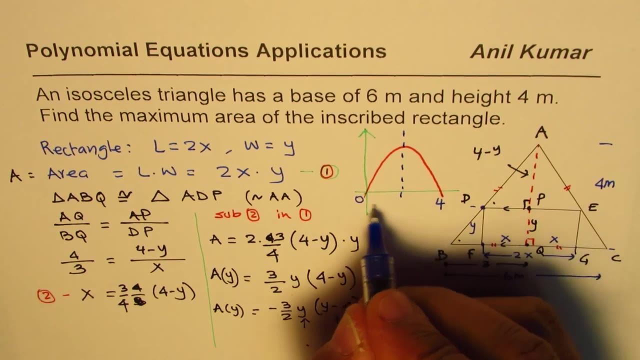 these zeros, as we notice here, will be at 0. because of this right And because of this factor, at 4,. how can I get maximum area? It should be at the axis. An axis will be midway, which is half of 0 and 4, which is 2, right. 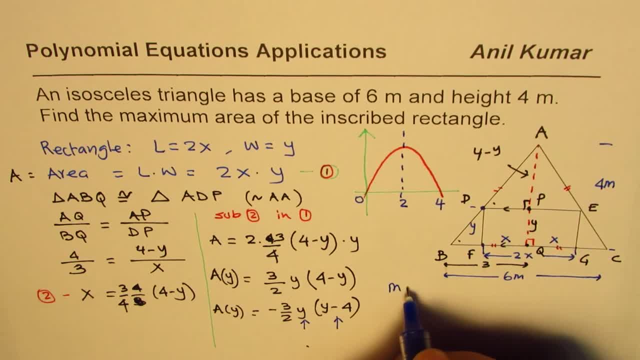 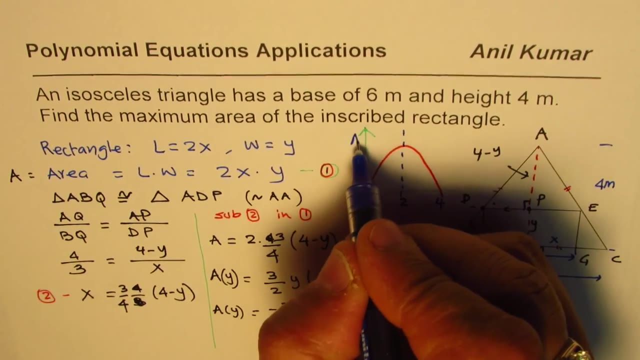 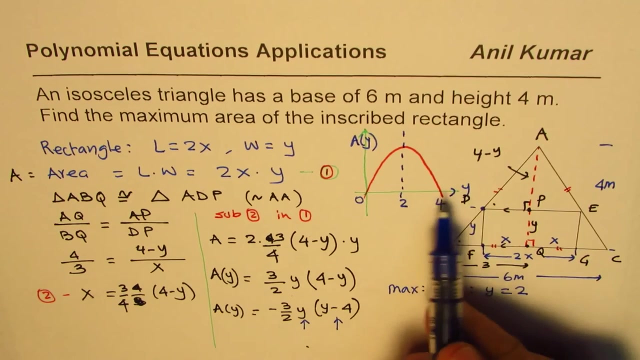 So what we find here is that maximum area is at the y value of 2,. right, See this y value, right? So in this case we are writing area as terms of y and we are actually writing y here. okay, This variable name is y. okay, Don't confuse with x and y axis. The 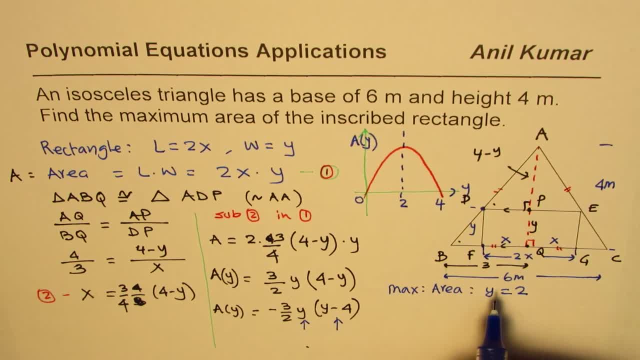 independent variable is y for us. So for y equals to 2, we get the maximum area. Now, if y is 2, what is the value of x? We can substitute here? right, We can find that value also. So y is 2,. 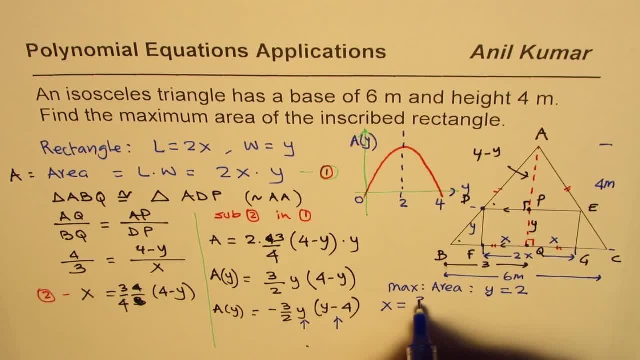 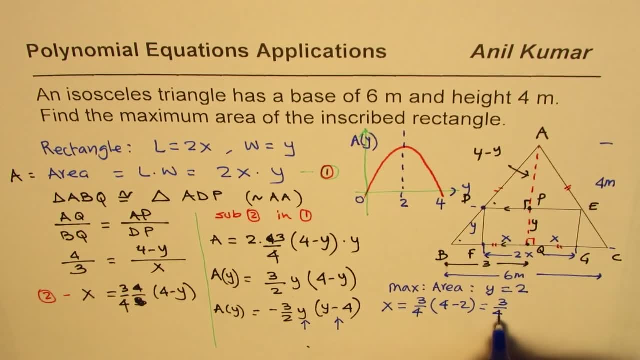 x is equal to 3 over 4 times 4, minus the y value, which is 2, which is 3 over 4, times 4 minus 2 is 2, right, So we could write this as 3 over 2.. That is x value. Now the question is: find the maximum area of the inscribed. 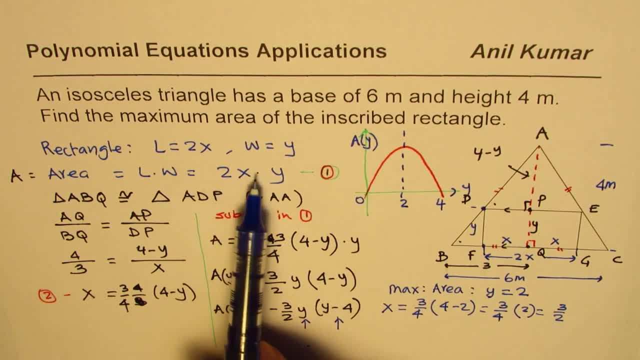 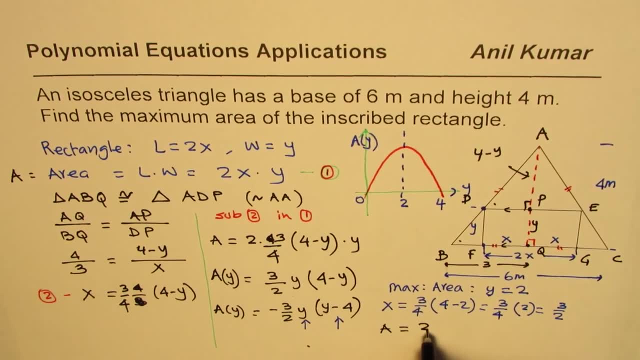 rectangle. So we got x and y values. We know the formula right, So we can write: the maximum area a is equal to 2 times the x value, which is 3 over 2, times the y value, which is 3 over 2,. 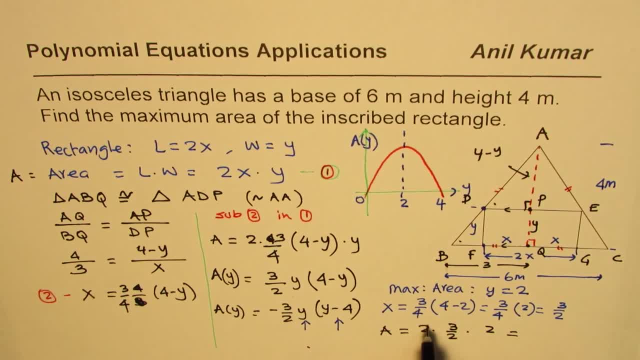 times the y value, which is 2, right, So that gives us 2 and 2 cancels 3 times 2 is 6.. The units are meters squared. Do you see that? So that is how we could find the maximum area. 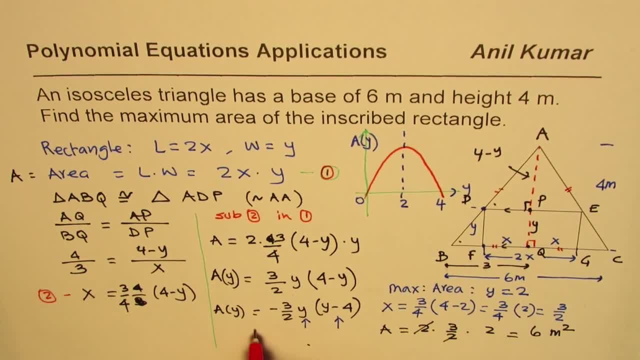 You could also substitute this value here and find maximum area for a, as the value in y is 2.. So if I substitute here, I get minus 3 over 2 times 2 times 2 minus 4.. Do you get it? 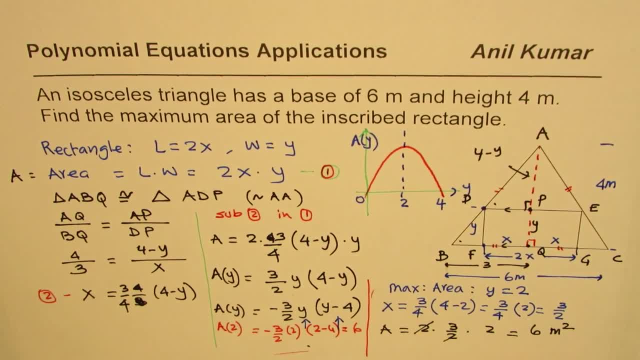 So minus 3 over 2, plus 2 minus n is also 6.. The same thing, So we could do it either way, right? So from here we know that the dimensions of the rectangle are 2 times x, right? So 2. 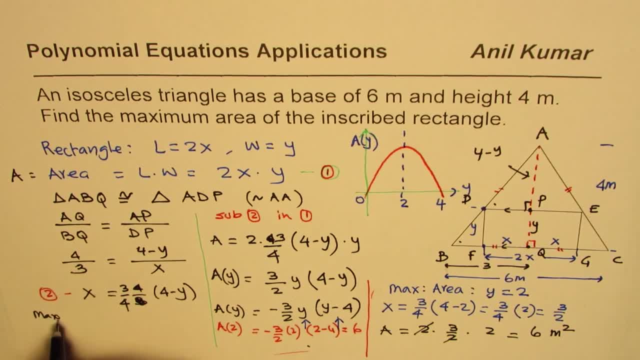 times x is 3.. So the maximum area- let me write maximum area- is 6 meters squared. We have not asked for the maximum dimensions, Sometimes it will be. So it will be 2 times the x value. So